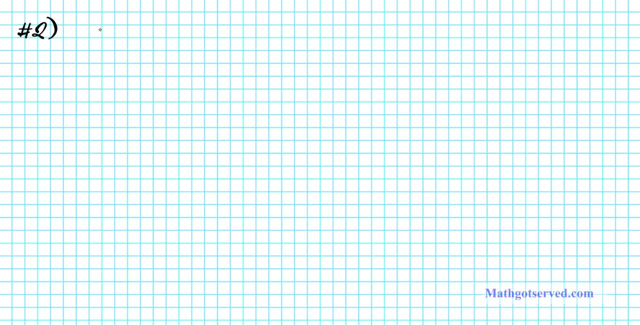 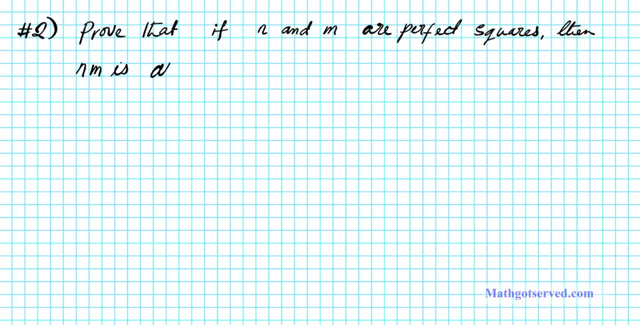 product n and m is also a perfect square. So this is what we are going to prove today. Okay, so first thing we are going to do, let's take a look at n and m. We are told that they are perfect squares. Now how can we capture that statement in a mathematical form, Can? 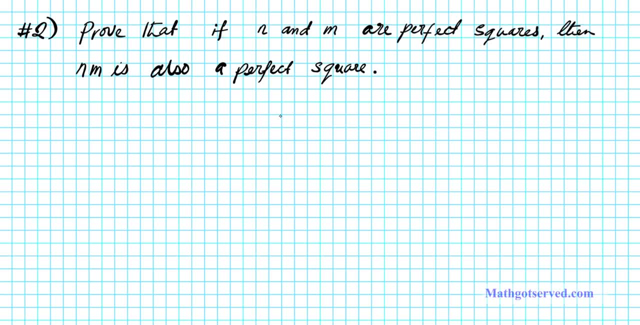 we write an equation using this fact And the answer is yes, Alright. so since we are asked to prove the following, So this is our proof right here, Let me delineate it so you know where I am starting from. Proof, since n and m are perfect squares, what does that? 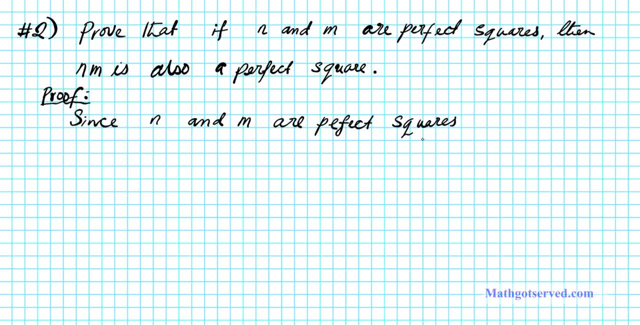 mean, Since n and m are perfect squares, then n is equal to a square. And since n and m are perfect squares and m is equal to b square for some integers- integers a and b. Okay, so any number that is a square can be expressed as any integer a square. For example, if you: 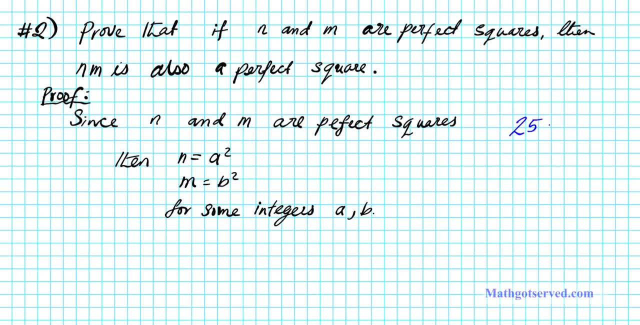 have 25,. 25 is a perfect square because it can be expressed as 5 square and you notice that 5 is an integer. So this is what is done. more than this. A has very few integers in the table and b has only five. It is very easy to integrate an integer in a question. 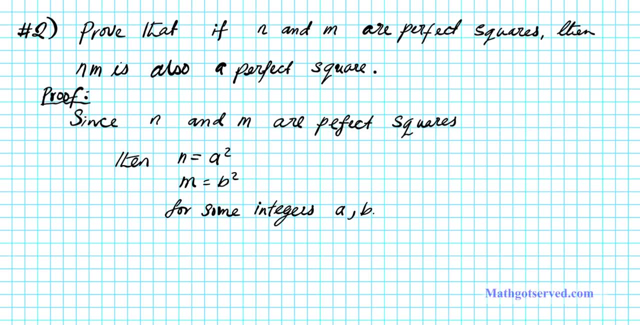 it is to be a square by definition. Okay, so let's go ahead and write that down, since n and m are perfect squares and n is equal to a square and m is equal to b square for some integers. a, b. by definition of a. 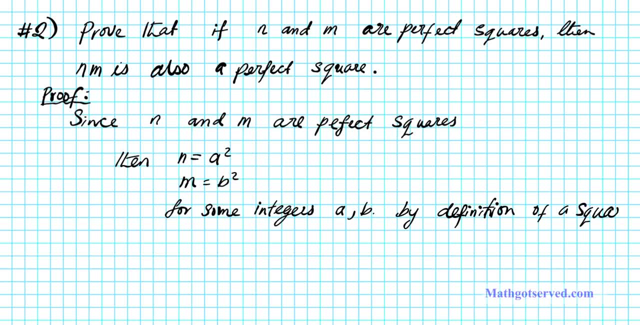 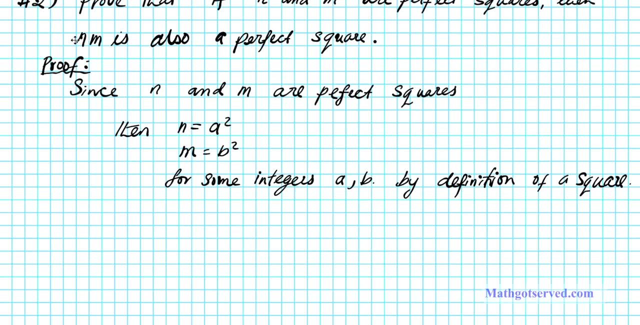 square. All right, so by definition, we can make these two statements. Now we have an equation that we can use to represent to find what the value of nm is. All right, so nm is simply going to be a square times b square. okay. 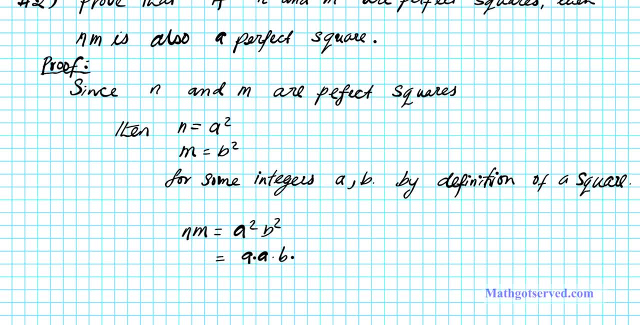 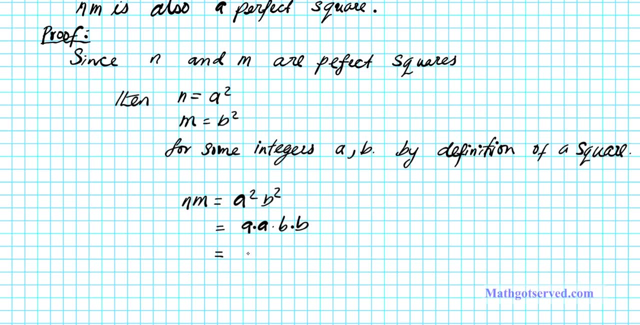 And then we can write this as a times a times b times b, using the properties of exponents. Now, what can we do? We know that multiplication commutes, So we can write it as a times b times a times b- commutative property. commutative property. 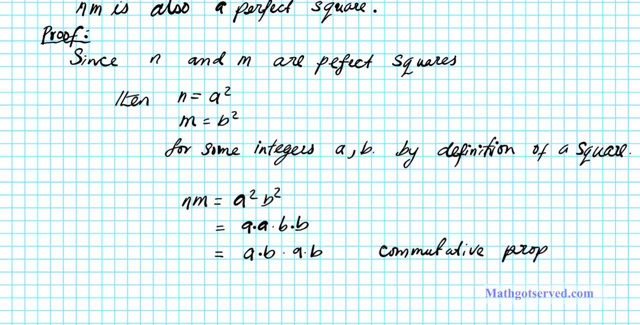 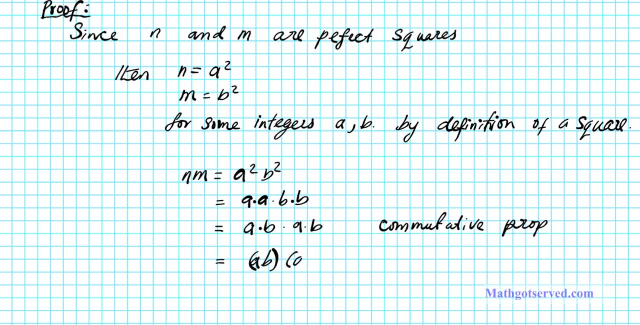 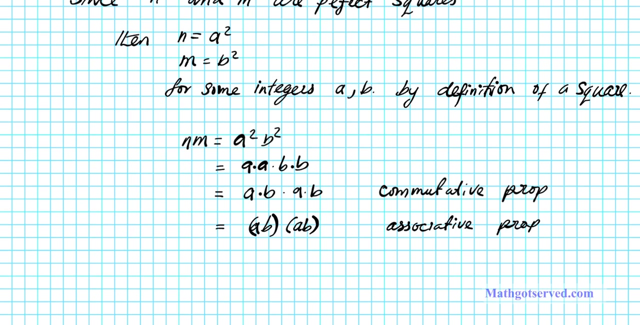 right there of multiplication, And then we can then associate them in this order: ab times, ab. okay, using the associative property of multiplication. Okay, So if you associate the multiplicands, you do not change the value of the product. It doesn't matter how you associate them, you still get the same answer. 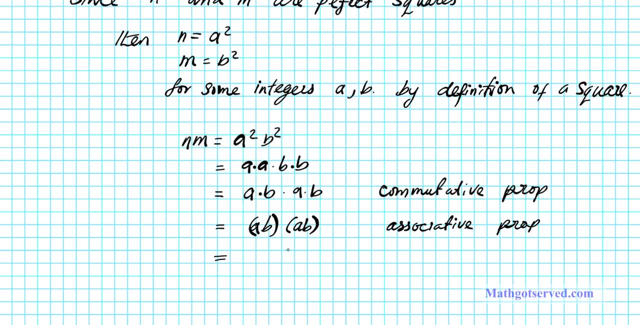 So we can associate them in this fashion. Now, using the properties of exponents, we are multiplying to identical bases. What do you do? You add the powers, right? So this is the same thing as ab square. So nm is equal to ab square. 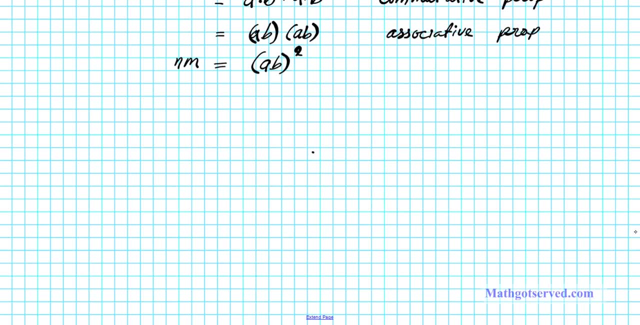 Now, what do we know about ab? That's the next question. Since a and b are integers, then what do we know about the product? The product is going to be an integer also by closure, right? So since a and b are integers, then ab is also an integer, because integers are closed. 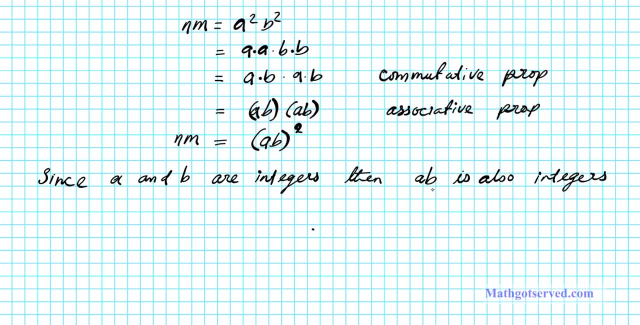 under multiplication. When you multiply integers, you get an integer. Okay, ab is also an integer, So let's make a substitution here. First of all, I would like to declare the variable I'll use in making my substitution. Let s equals ab. all right for some integer s, for some integer s. 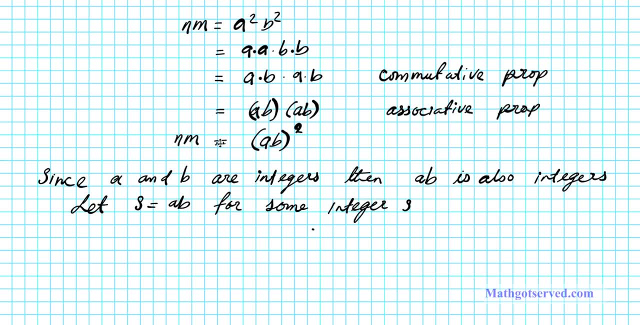 So if I make that substitution of the value of ab, which is s, into this equation and m, here, I will have: nm is equal to. instead of ab, I will have nm. Okay, Okay, So I will have: nm is equal to s? square.